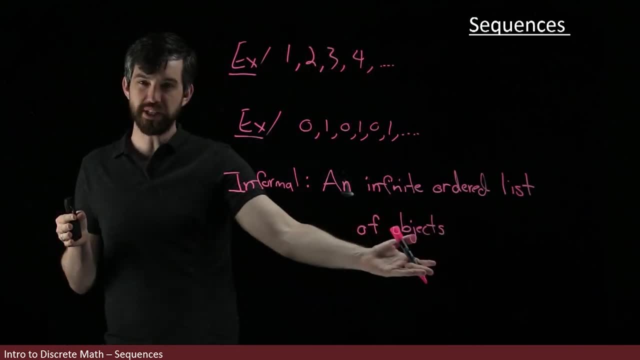 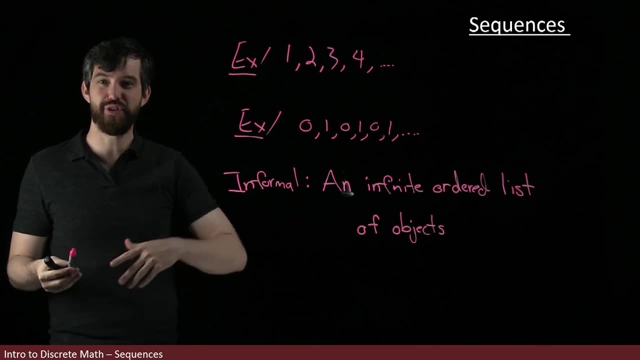 Note that I don't do this. I don't put numbers here. The objects could be all kinds of weird mathematical things, although we normally deal with numbers. So, for example, I could have an ordered list of functions or an ordered list of sets or all kinds of different objects. 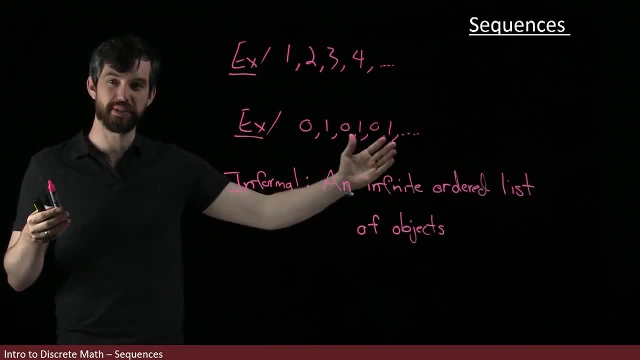 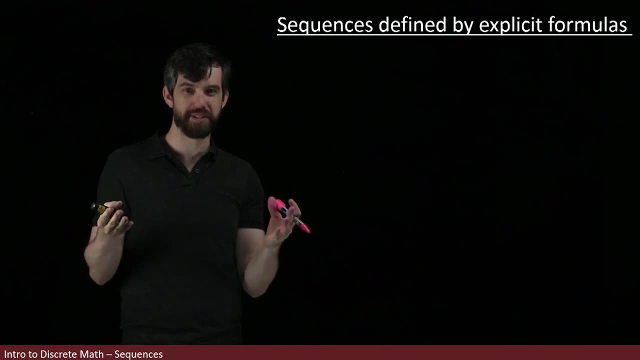 But for the most part we'll be dealing with an ordered list of numbers. In the previous examples we sort of picked up the pattern of the sequence just by looking at the first couple terms, But sometimes what we do is write explicitly down: 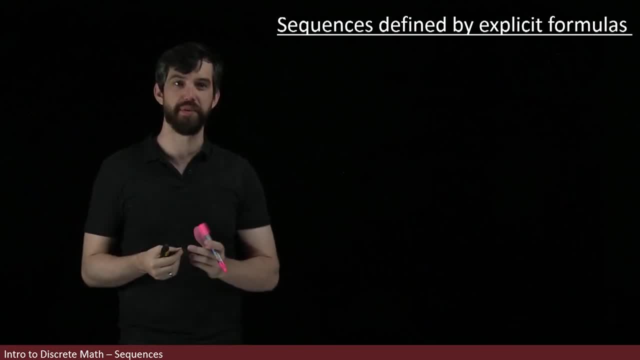 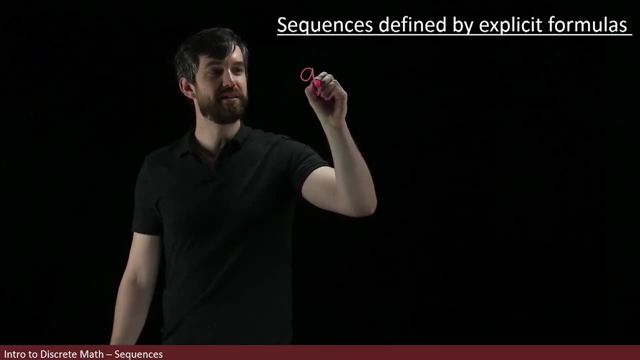 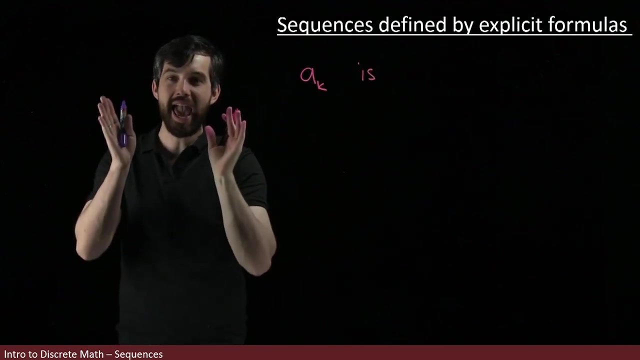 what the formula for the particular sequence is going to be. So, in order to do this, I need a little bit of notation: which is the symbol- a sub k- And what a sub k is going to refer to. this is going to be the kth term of my sequence. 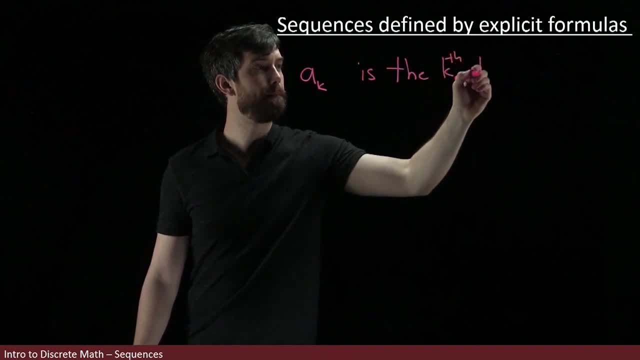 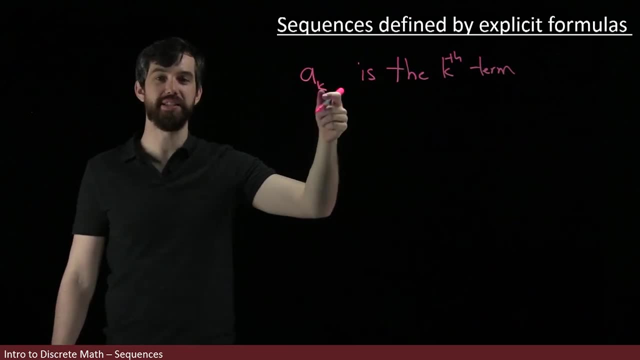 So is the kth term. So, for example, a sub 1 is the first term, a sub 2 is the second term and generally a sub k is the kth term. So if I want to have an explicit formula, 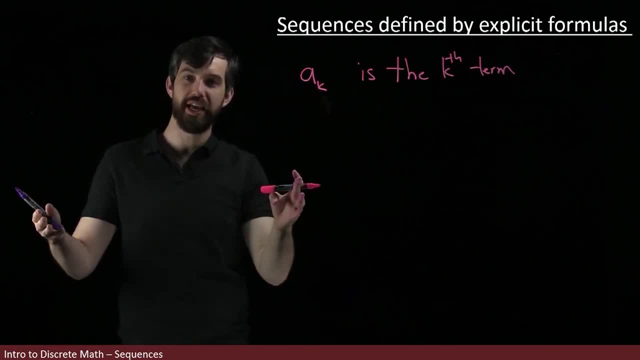 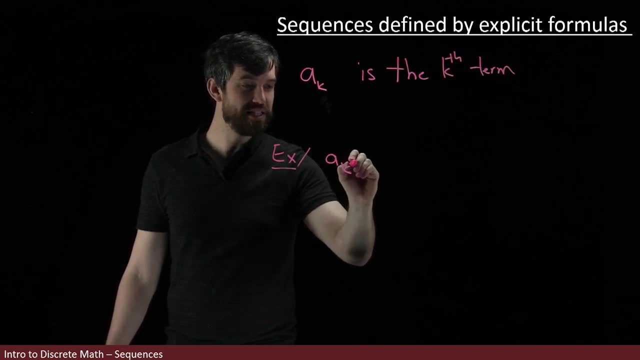 what I need to do is I need to tell you what are all of the a? k's. So I want to give as an example this: I'm going to claim that a sub k is just equal to k. Okay, so this is like the simplest one that I can imagine. 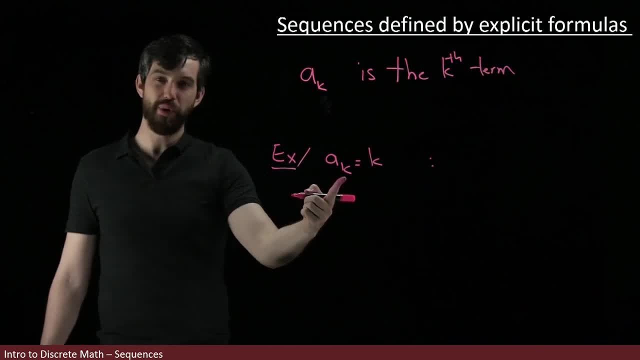 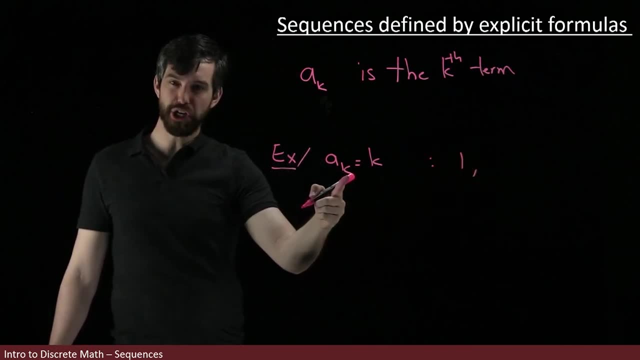 So if I want to think about what this means for my sequence, then. so what I'm saying is that a sub 1,- the first term, is just 1.. So that's this, And then a sub 2,, which is my second term, is just 2.. 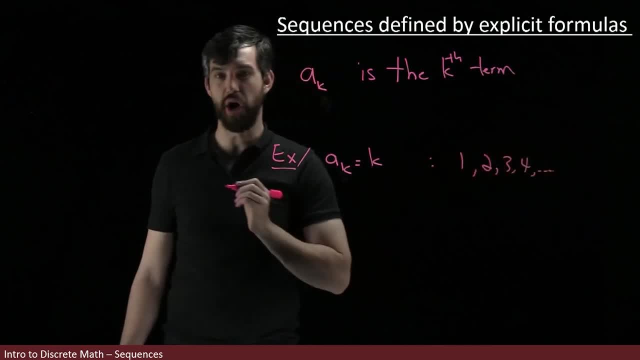 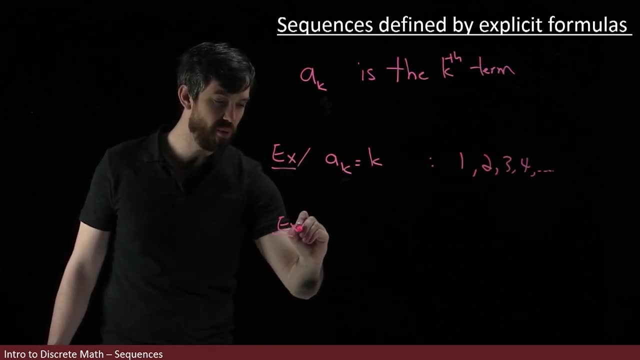 So 1,, 2,, 3,, 4, and continues on. This is indeed just precisely the sequence that we saw before, But I can do much more interesting and convoluted ones here. So, for example, how about this? 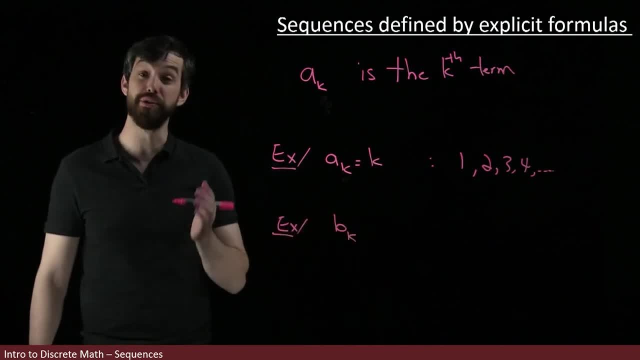 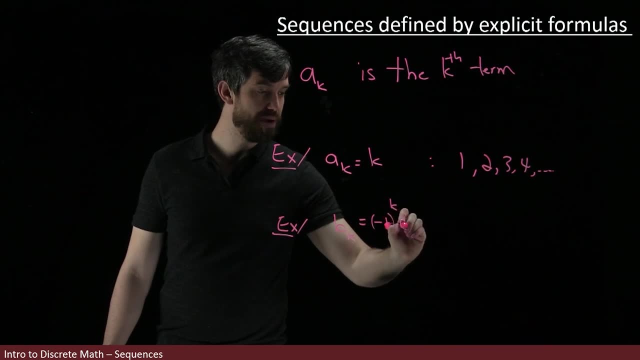 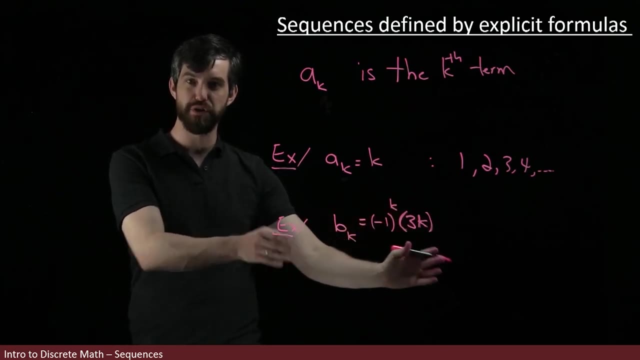 I'll use bk this time because I'm doing a new sequence. I'm going to say it is minus 1 to the power of k multiplied by 3k. Okay, so let's try to write out the first few terms for this sequence. 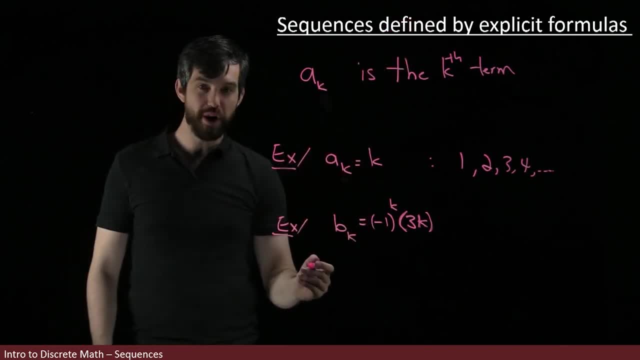 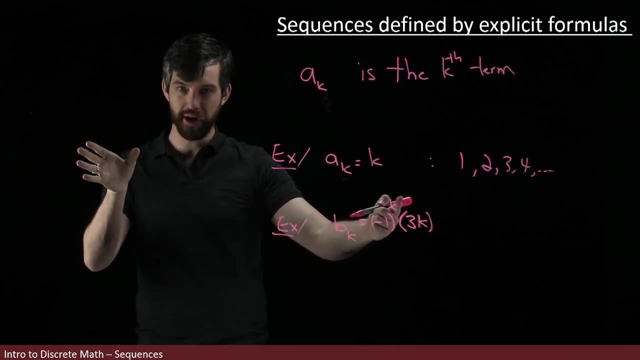 which has been defined by an explicit formula. So the first one, if I look at the first term, is k equal to 1.. So minus 1 to the k, that's going to be just a minus 1.. And then 3 times 1, so the first term is going to be minus 3.. 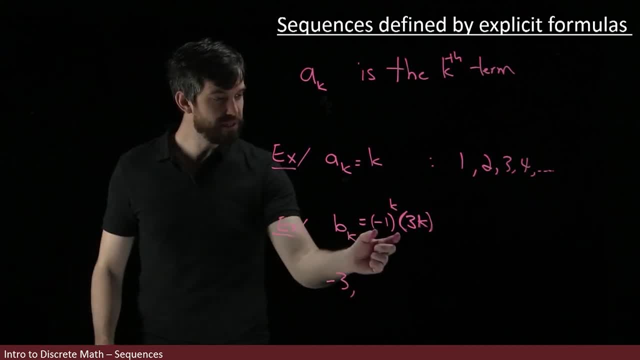 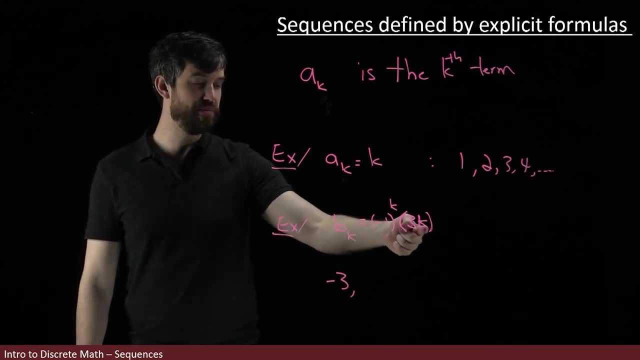 And then I'm going to look at the next term. So this is k equal to 2.. Now it's minus 1 squared. Minus 1 squared is positive 1, so there's no negative sign. And then 3 times 2 is going to be 6.. 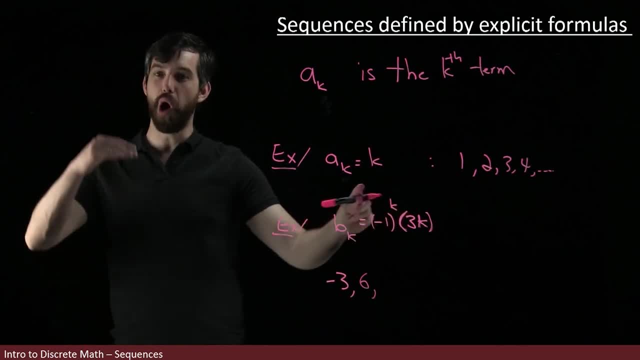 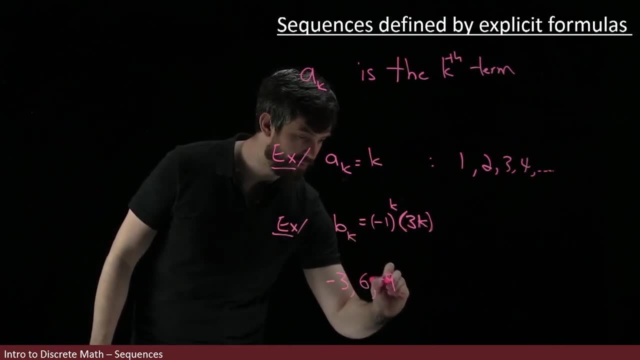 Okay, I'll look at my next one: Minus 1, cubed. it's an odd power now, so this is going to bring out a minus 1.. And then 3 times 3 is going to be 9, so minus 9.. 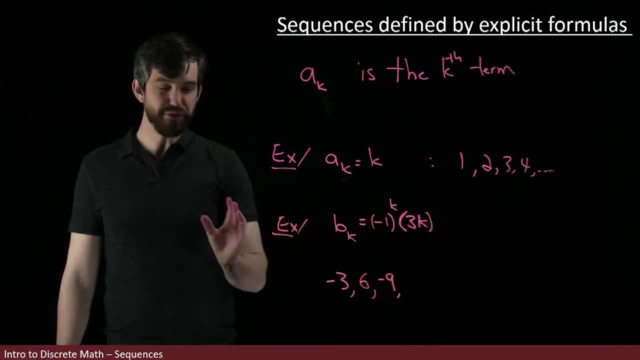 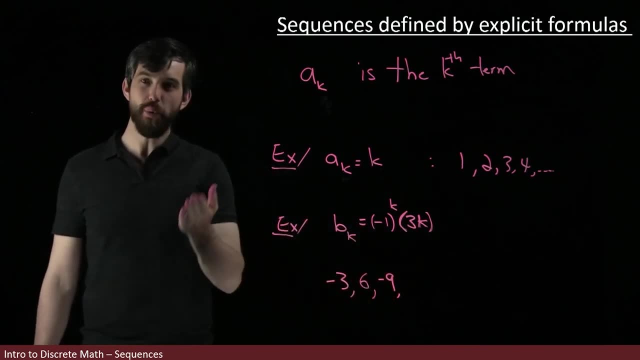 So there's a couple different components to think about here. First of all there's the k, which we've seen before. So the k sort of has like an underlying 1,, 2,, 3, 4.. But then that 1, 2, 3, 4 gets multiplied by this extra 3.. 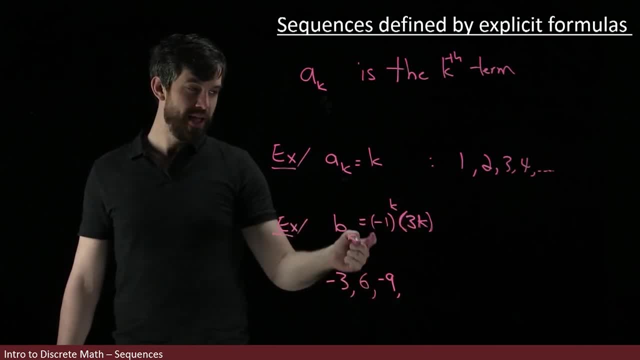 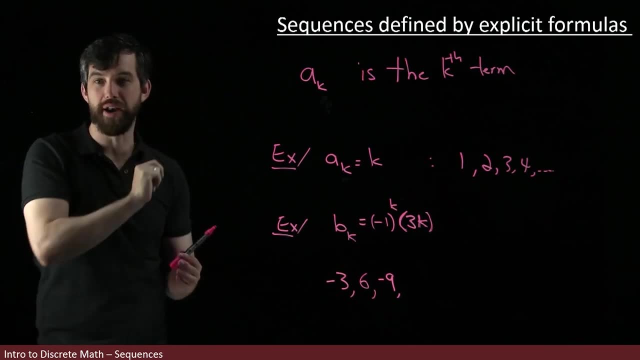 So 1, 2, 3 turns into 3,, 6, 9.. And then the interesting one is this: minus 1 to the k, Because minus 1 to the k depends on whether that k is even or odd. 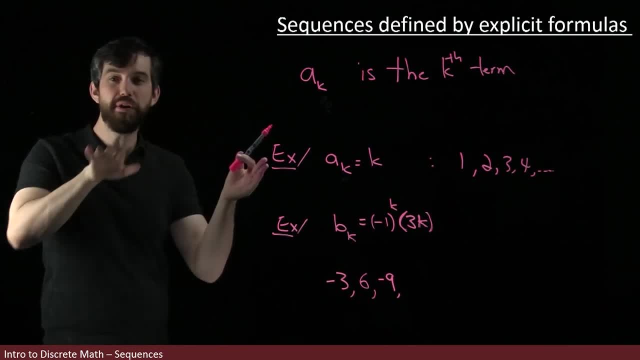 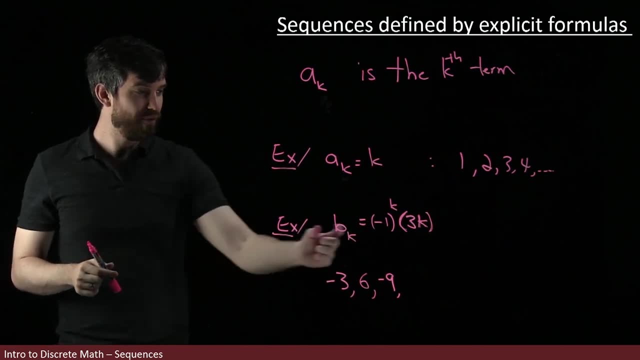 When it's even minus 1 to an even power, all of those are going to be just giving out the value of 1.. Minus 1 squared is 1.. Minus 1 to the fourth is 1.. But if I take the minus 1 to an odd power, 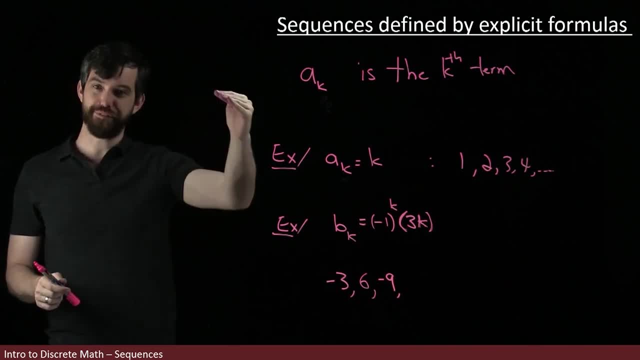 like minus 1 to the 1, or minus 1 to the 3, or minus 1 to the 5, all of those are going to give you a negative sign. So, as my k goes up, 1,, 2,, 3,, 4,. 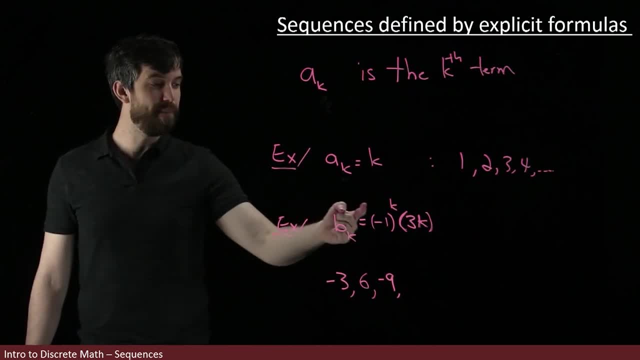 it keeps alternating between whether it's odd or even So. I get a minus sign and then I don't get a minus sign. Then I get a minus sign and then I don't get a minus sign. So, without even looking at it, I can look at the next one. 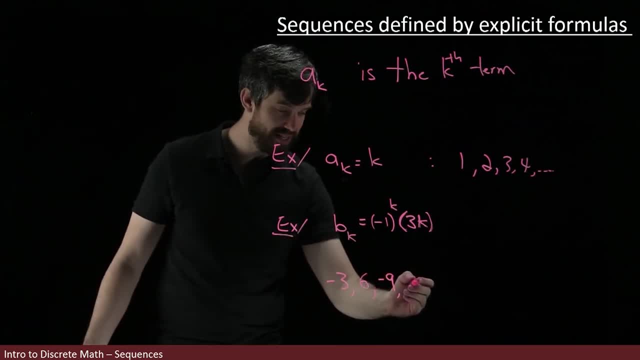 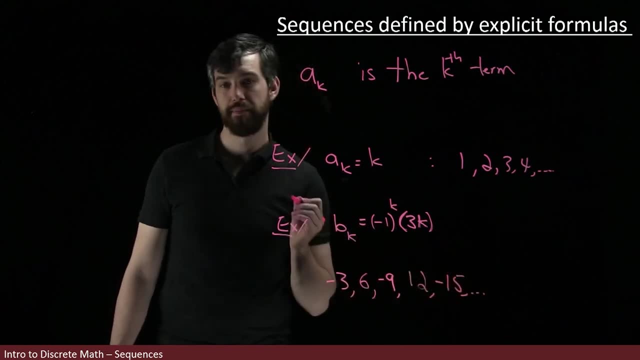 and when I go minus, no, minus, minus, it's going to have no minus in the next one and it's going to be 4 times 3,, so 12.. And then the next one would be minus 15, and so on. 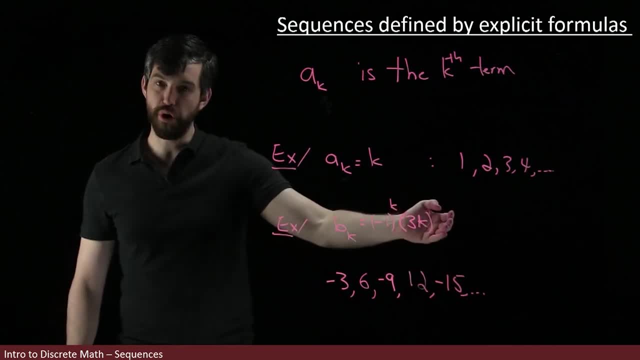 So this problem can work two different ways. I can either give you the formula and you can write down the first few terms, or I can give you the first few terms and you can write down what the formula's going to be.